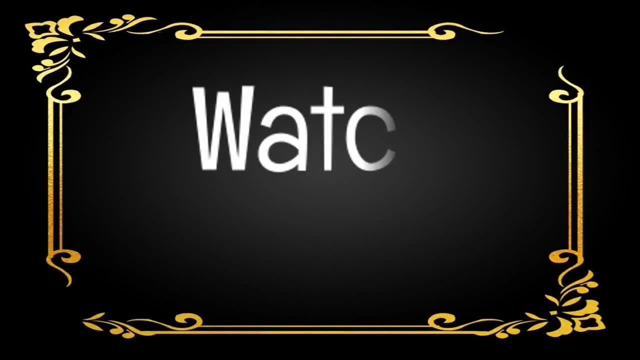 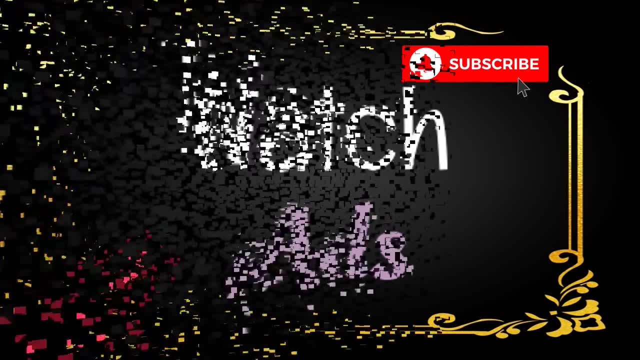 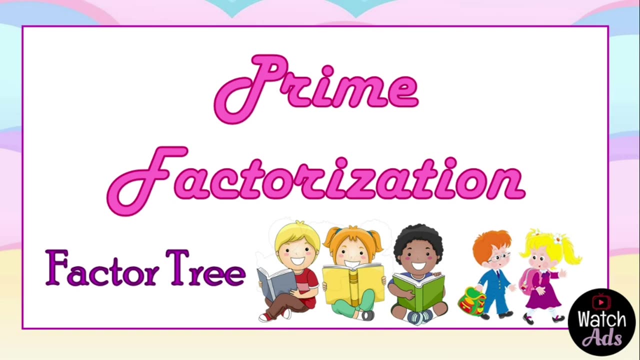 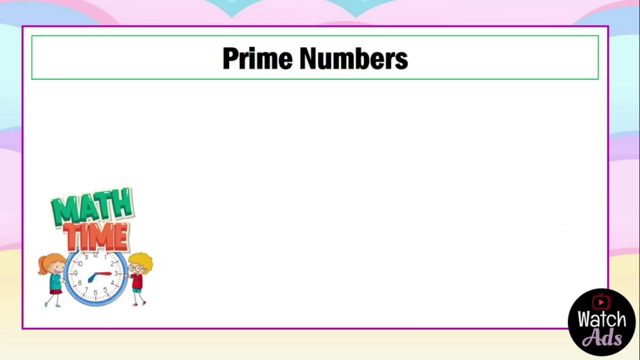 Hello everyone and welcome back to my channel. For this video. we are going to talk about prime factorization or the factor tree. In my previous video we have discussed about prime and composite numbers. If you haven't watched that video yet, please click the suggested video above. 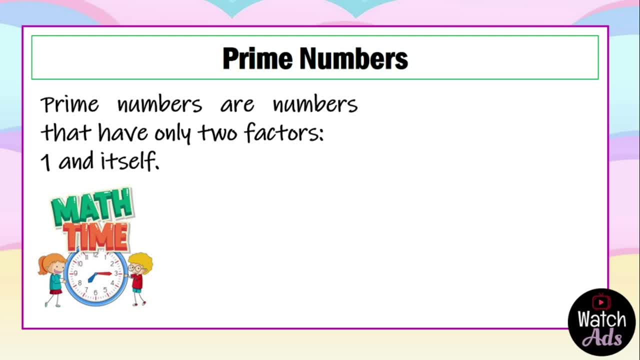 Remember, prime numbers are numbers that have only two factors, that is, 1 and itself. Examples we have 3.. 3 is prime because it only has two factors: 1 and 3.. 59 is also prime because it only has two factors: 1 and 59.. And 97 is a prime number because it only has two factors. 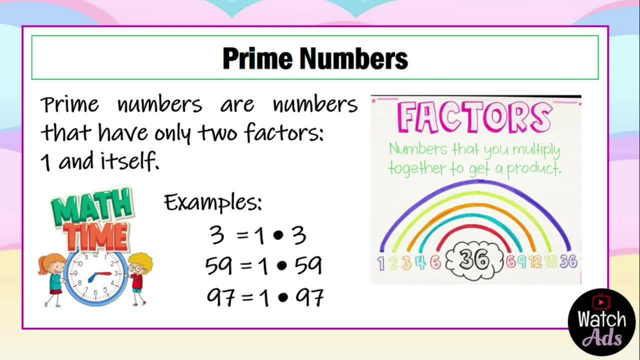 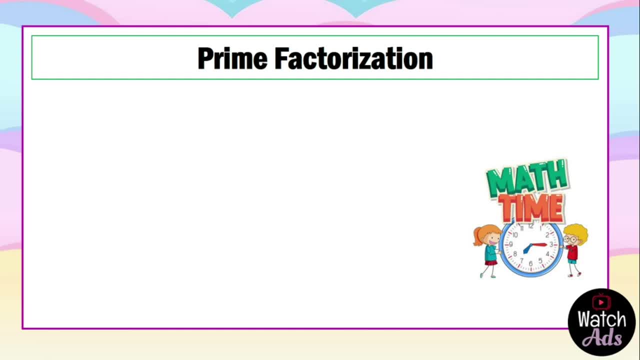 1 and itself. Remember factors are numbers that you multiply together to get product. In prime factorization you are given a composite number. The thing you have to do is to factor out the composite number and you should end up with prime factors only. Remember there are four. 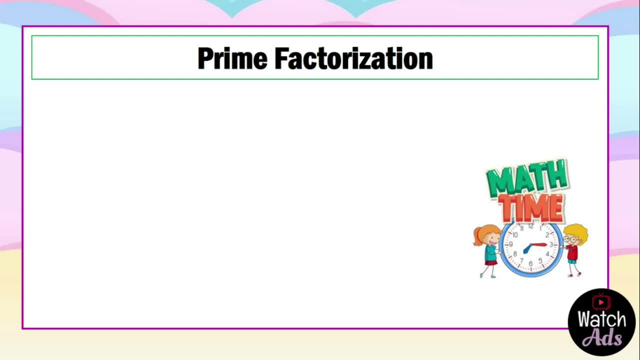 single-digit prime numbers that are 2,, 3,, 5, and 7.. These are the most commonly used prime factors. Let's have an example. What are the prime factors of 16?? 16 is a composite number, so we can factor. 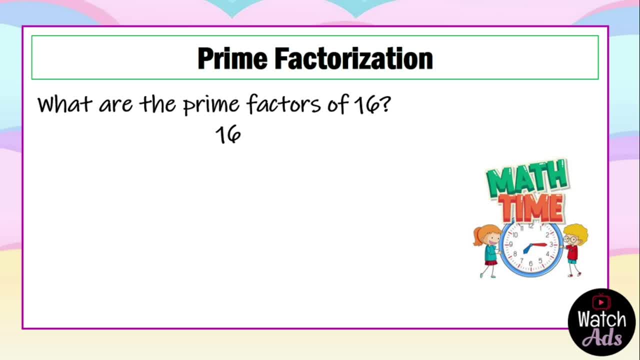 that out. First, you think of two numbers that if you multiply together gives a 16. For an instance, let's have 4 times 4, because 4 times 4 is equal to 16.. Now we write them down: 4 and 4.. Check if 4 is a prime number, 4 is a composite number, so we can. 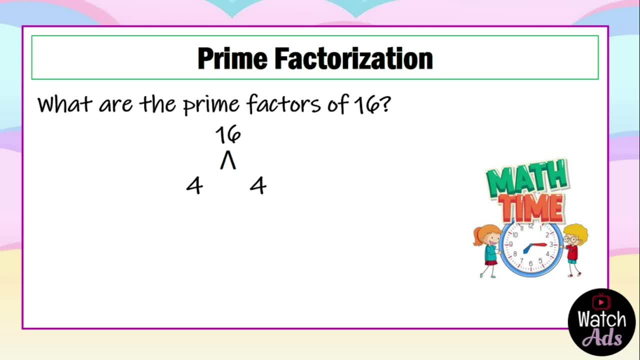 still factor that out. What are the factors of 4?? We can have 1 and 4 or 2 and 2.. But remember we should end up with prime numbers and 1 is not a prime number. So let's have 2 multiplied by 2.. 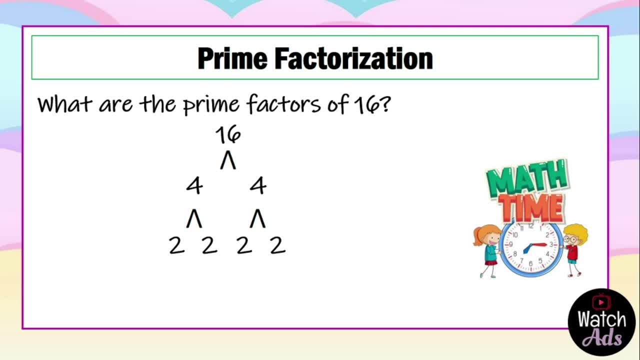 And then we write them down. finally, we check if the numbers are prime numbers and 2 is a prime number. so these are our prime factors. let's write them down. 16 is equal to 2 times 2 times 2 times 2 and that is our final. 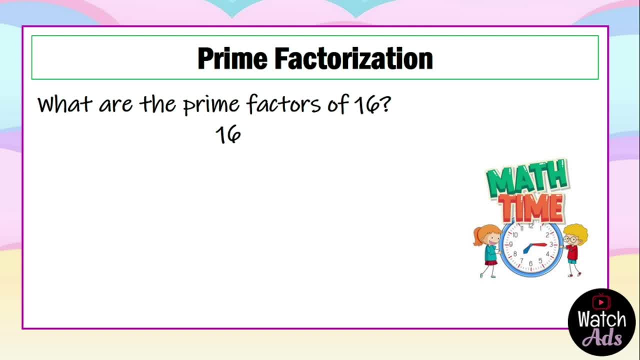 answer. now what if you think of other factors of 16, aside from 4 and 4? let's try 8 and 2. write down 8 and 2. 2 is a prime number. so we end up there now. we factor out 8, think of two numbers, we multiply. 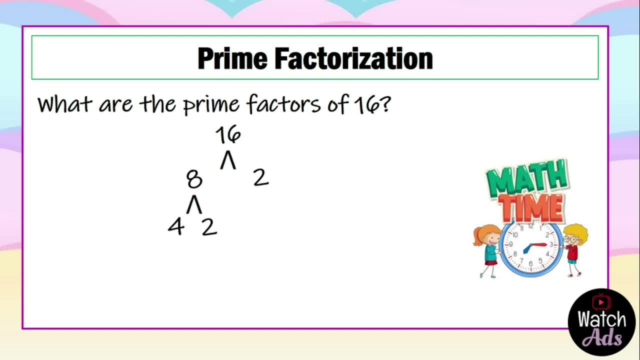 together gives us 8. yes, we have 4 and 2. 2 is a prime number. so we end there. we factor out 4. we have 2 factors 2 and 2. now we end up with prime factors. let's write down our answers: 16 is equal. 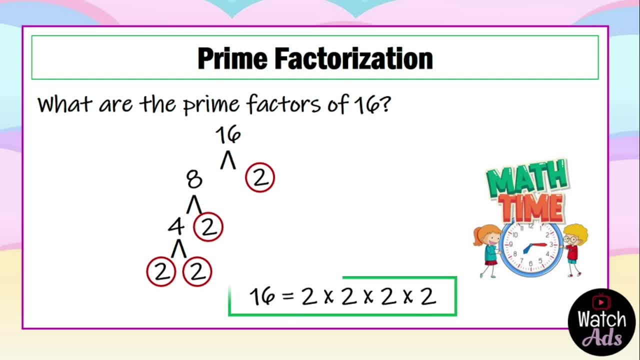 to 2 times 2 times 2 and that is our final answer. and if we are going to try to compare with our previous solution, we still end up with the same answer. let's have another example: prime factors of 30. you write 30 and we factor it out. let's have 6 times 5. 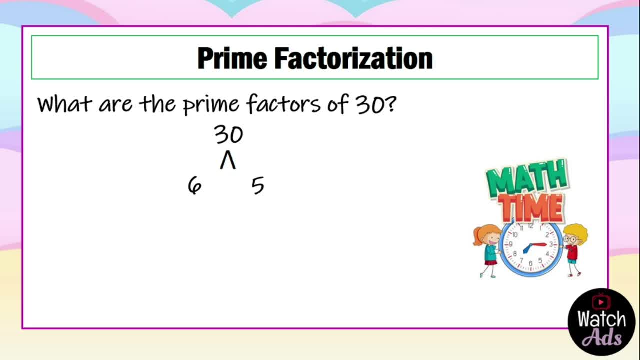 and then we write down: 5 is a prime number, so we end there: 6 is a composite number, so we can still factor that out. multiply 3 and 2 it gives a 6, so we write them down: 3, 2 and 5 are. 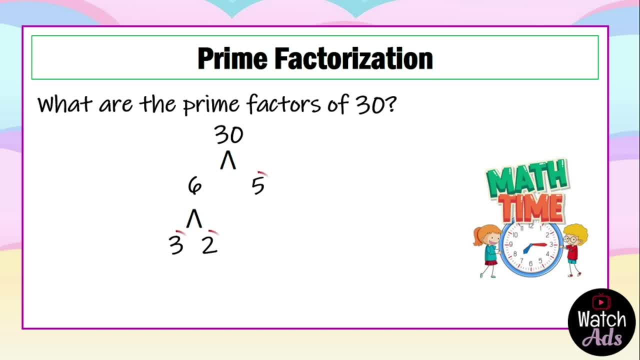 prime numbers. so those are our final answers and then we write it down: 30 is equal to 5 times 3 times 2, and that is our final answer for our last example. let's try 42. 42 is a composite number. we it out. Let's think of two numbers that if we multiply together gives us 42.. Let's try 6 and. 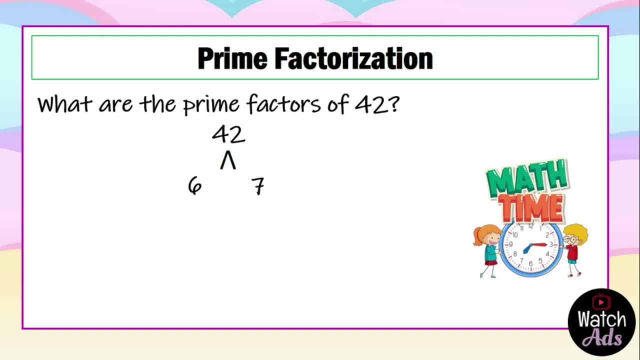 7.. 7 is a prime number, so we end there. We factor out 6.. We have factors 3 and 2.. 3,, 2, and 7 are prime numbers, So this ends our factor tree. Encircle them and write them down. 42 is equal to.